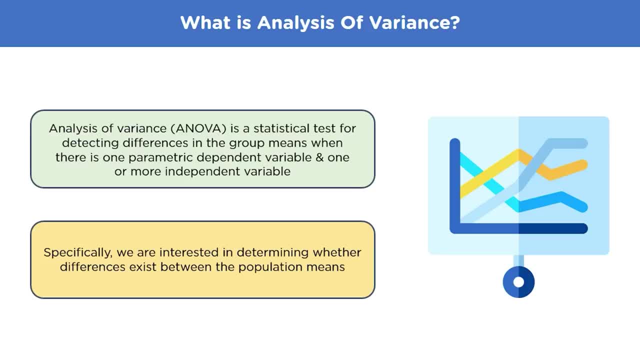 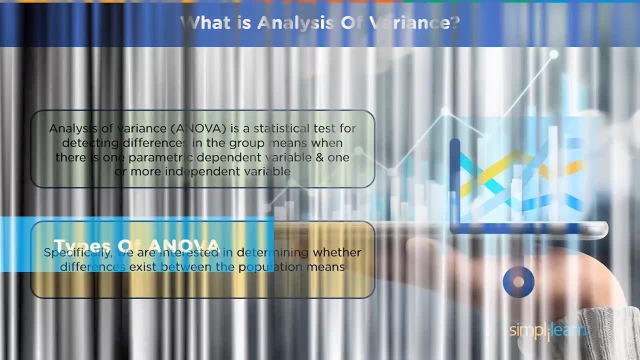 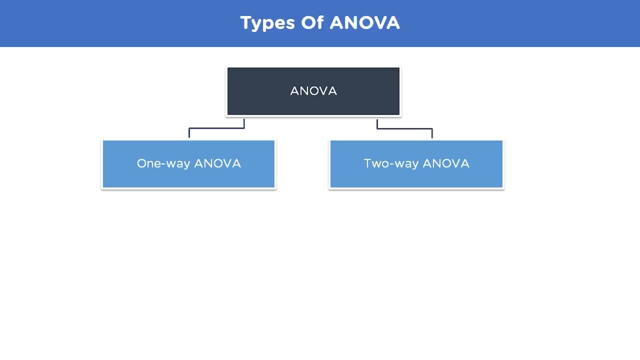 are equal. In a regression study, analysts used the ANOVA test to determine the impact of an independent variable onto the dependent variable. So what are its types? There are basically two types of ANOVA, which is a one-way ANOVA. 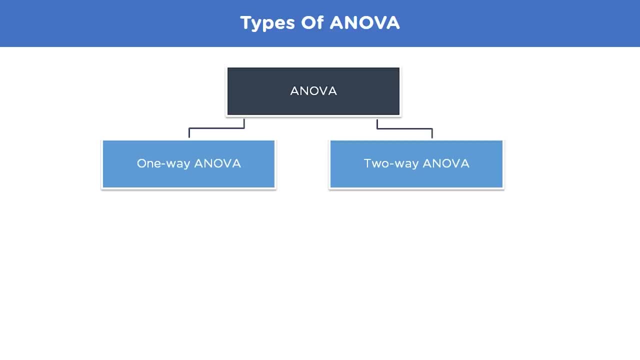 and a two-way ANOVA. When we are comparing more than three groups based on one factor variable, then it is said to be a one-way analysis of variance. For example, if we want to compare whether or not mean output of three workers is the same, based on the working hours. 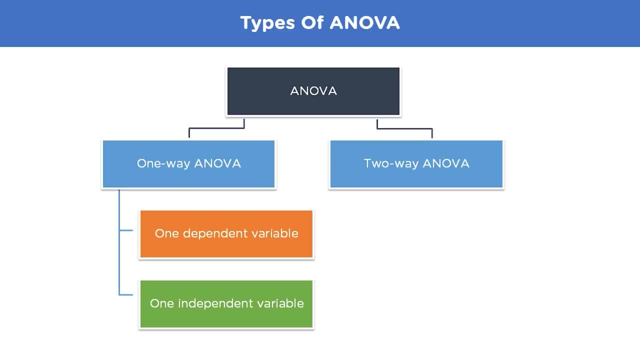 of the three workers, we will use a one-way ANOVA. When factor variables are more than two, then it is said to be a two-way analysis of variance. For example, based on working conditions and working hours, we can compare whether or not. 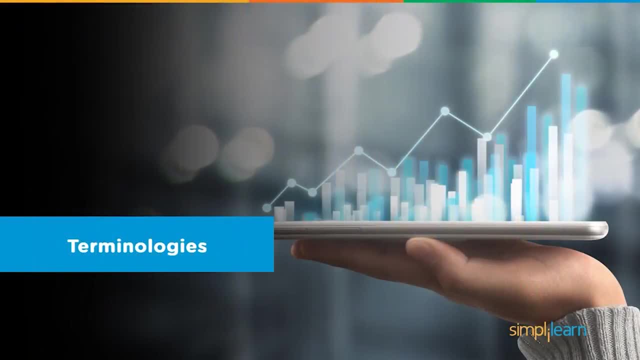 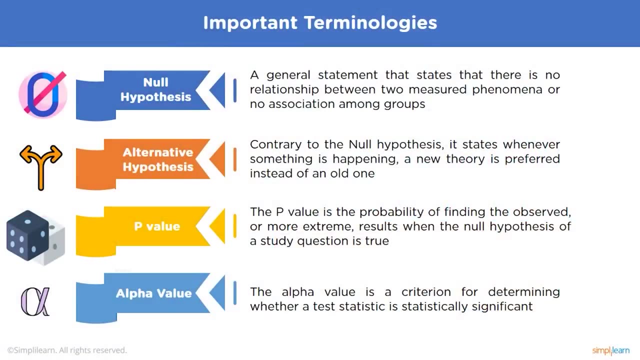 the mean output of three workers is the same. Now let's discuss some key terminologies used in ANOVA. We'll start with a null hypothesis. The null hypothesis is the assumption that an event will not occur. A null hypothesis has no bearing on the studies. 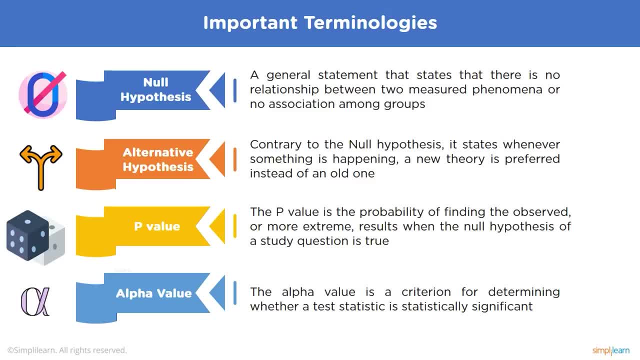 outcome unless it is rejected. Alternative Hypothesis. The Alternative Hypothesis is the logical opposite of the Null Hypothesis. The acceptance of the Alternative Hypothesis follows the rejection of the Null Hypothesis. H1 is the symbol for it. 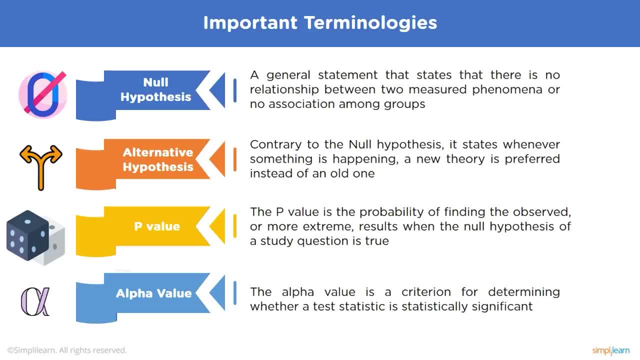 P-Value. In statistics, the P-Value, also called Probability Value, is the probability measure of finding the observed or more extreme results. when the Null Hypothesis of a given statistical test is true, The P-Value is the primary value used to quantify the statistical significance of the result. 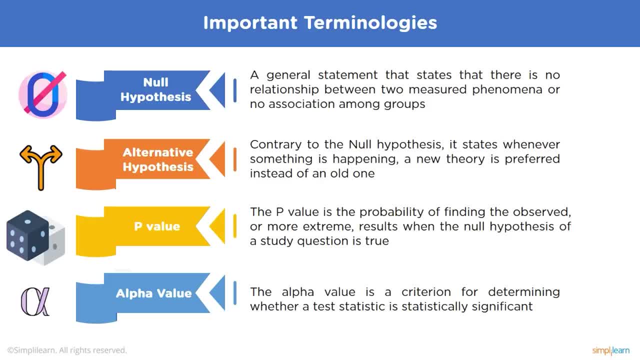 of a hypothesis test. Now let's move on to Alpha-Value. The Alpha-Value is the criteria for determining whether a test's statistics is statistically significant or not. This test provides the P-Value, which is the probability of observing results as extreme as those in the data, assuming the results are truly due to chance alone. 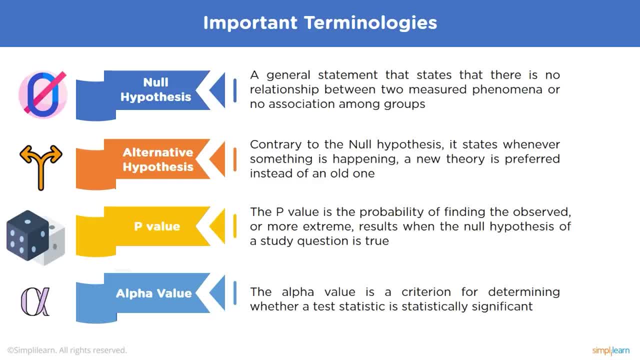 An Alpha-Value of 5% or lower is the probability of observing results as extreme as those in the data. assuming the results are truly due to chance alone, An Alpha-Value of 5% or lower is often considered to be statistically significant. 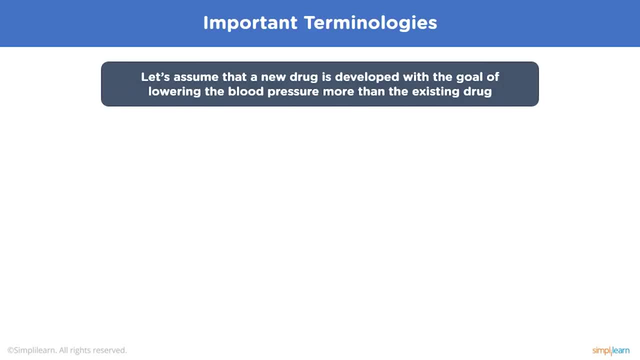 Now let's try to understand these terminologies by taking an example. Let's assume that a new drug is developed with the goal of lowering the blood pressure more than the existing drug. So in this case, a Null Hypothesis will be that a new drug doesn't lower the blood. 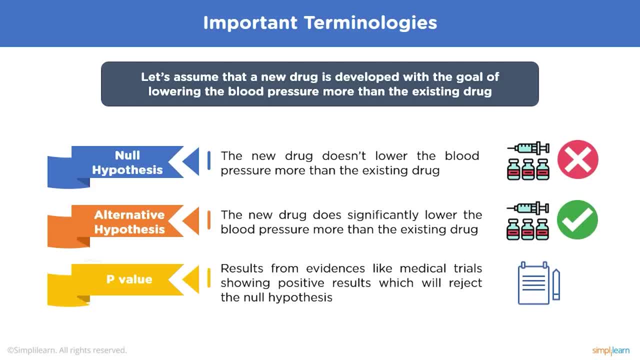 pressure more than the existing drug. The Alternative Hypothesis will be that a new drug does significantly lower the blood pressure more than the existing drug And the P-Value will be the result from evidence like medical trials showing the positive results, which will reject the Null Hypothesis. 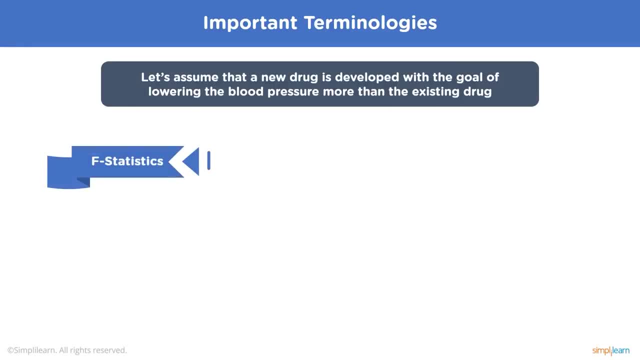 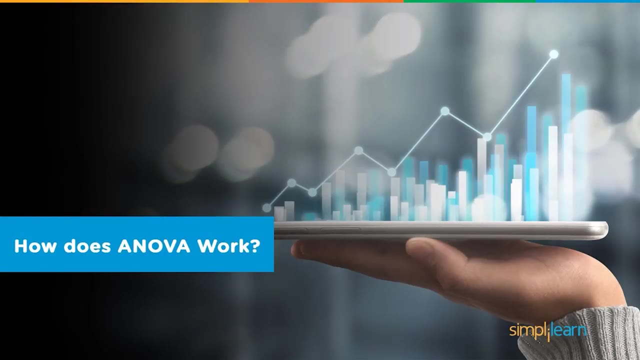 The S-Statistic will be the extent of difference between the means of different medical trials. the sum of squares will be the variation from the mean of different trials. The mean will be the average of all the results from evidence studies like medical trials. Now let's understand the co-concept between how the ANOVA works. 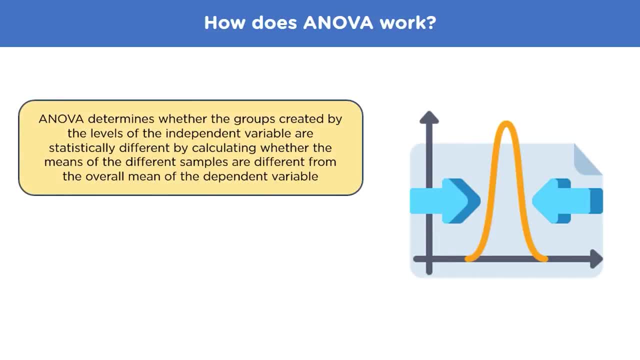 The oneway ANOVA compares the means between the groups you are interested in and distinguishes whether any of those means are statistically significantly different from each other. Let's simply do the Specifically. it tests the null hypothesis. If any of the group means is significantly different from the overall mean, then the null. 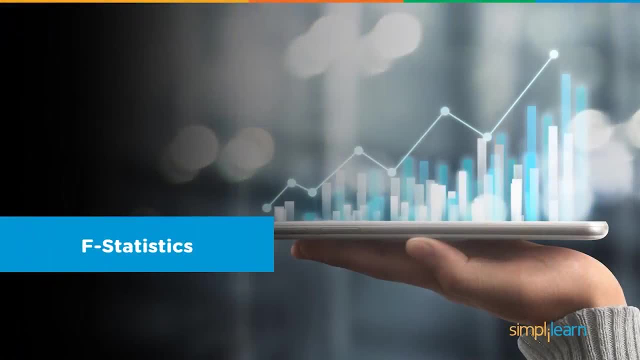 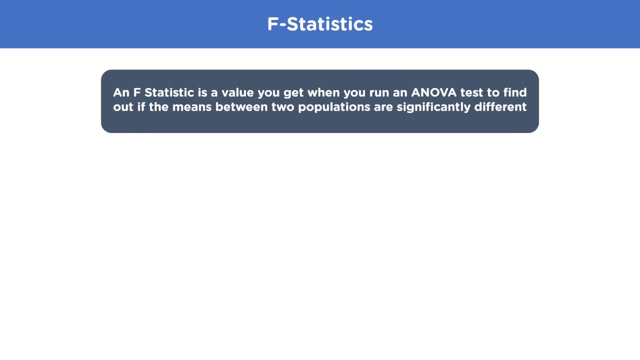 hypothesis in this case will be rejected. Now let's discuss the term F-statistics, which is very much used in the analysis of variance. F-statistics or F-ratio is a statistical measure that tells us about the extent of difference between the means of different samples. 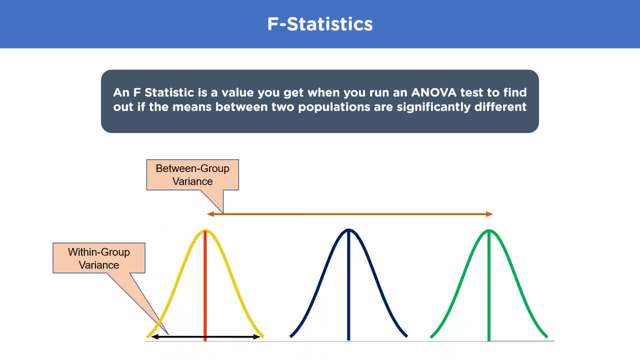 Lower the F-ratio, the closer are the samples to the means. If you have three different data sets, then this part will be the within-group variance, that is, the variance between the samples. This line will be the variance between the means of the different samples, which is also 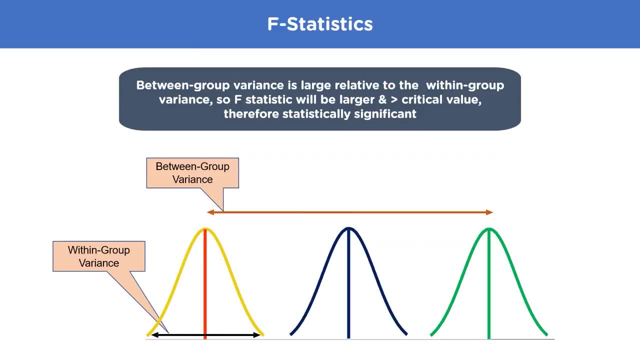 called between-group variance. If the between-group variance is large relative to the within-group variance, the F-statistic will be comparatively large to the critical value and therefore will be statistically significant. Now that we have covered almost all the theory regarding the ANOVA, let's try to understand. 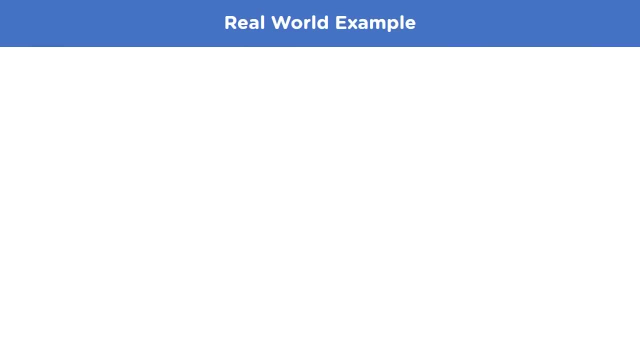 how this is used in a real-world example. Suppose you are a marketing manager of the product company. Your team has recently launched three new advertisements and you want to know if the three different types of advertisements affect mean sales differently. So how can you do that? 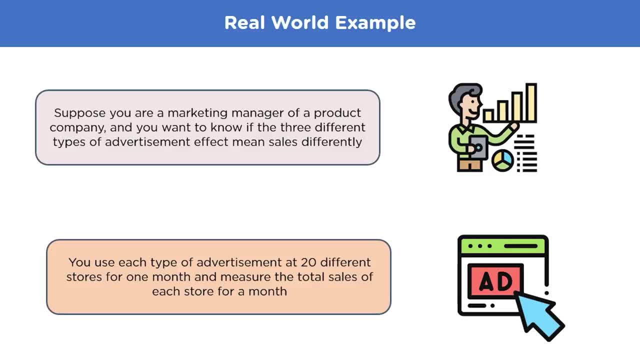 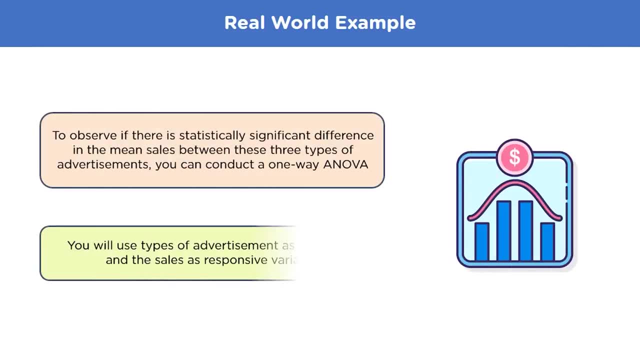 You will use each type of advertisements at 20 different stores for one month and then measure the total sales of each store for a month To observe if there is statistically significant differences in the mean sales between these three types of advertisements. You will conduct a one-way ANOVA. 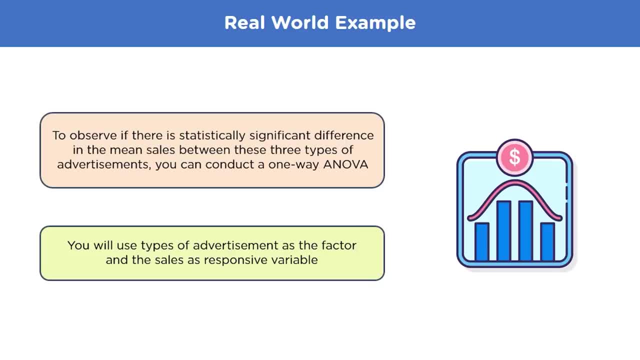 For calculating the ANOVA. you will use the type of advertisement as a factor and the sales as a response variable. Now that we have covered all the topics in ANOVA and have understood how it is used in a real-world example, let's see how you can run an ANOVA test in Excel. 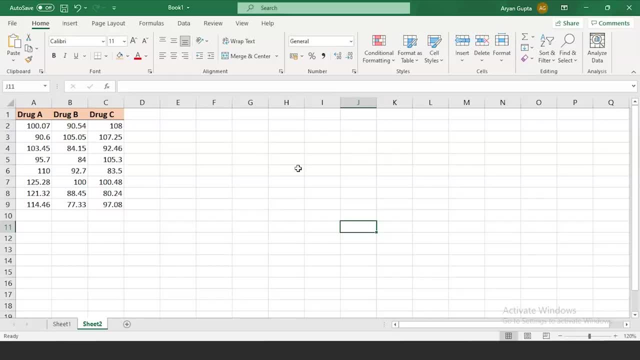 Suppose you are a research scientist and you want to perform clinical trials to study the effectiveness of three drugs developed by three healthcare companies to cure a certain disease. Anova represents the time taken to cure the disease for different patients when they consume either drug A, B or C. The time is represented in terms of total hours and minutes. 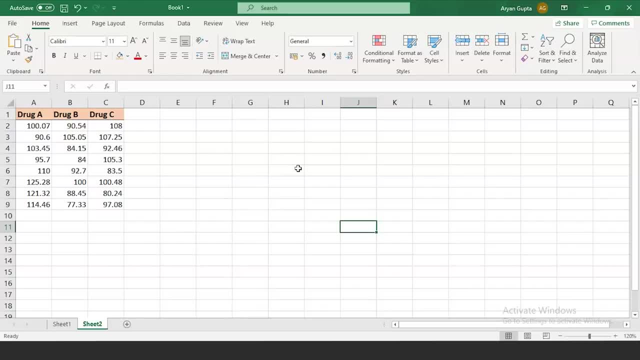 At the 0.05 level of significance, ie the alpha value. we need to test whether the mean time for the three drugs to cure the disease is equal. So how can you do that? We will first move on to the data tab and then click data analysis. 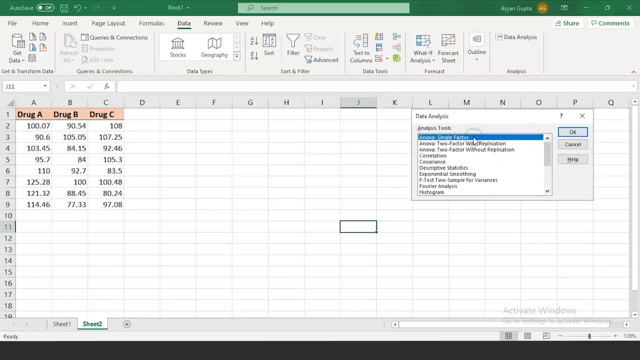 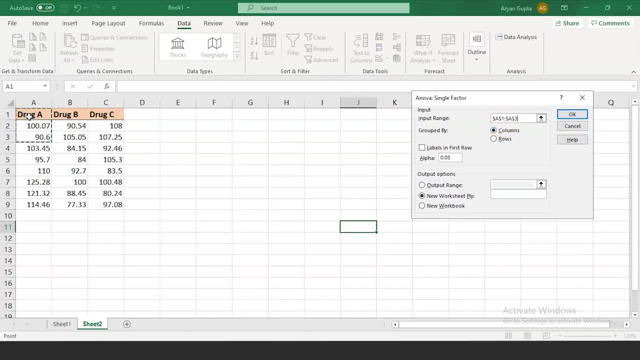 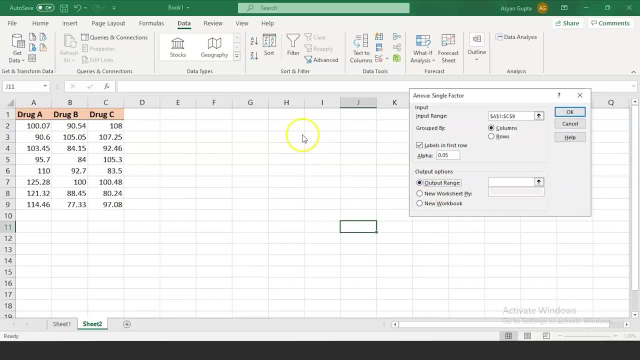 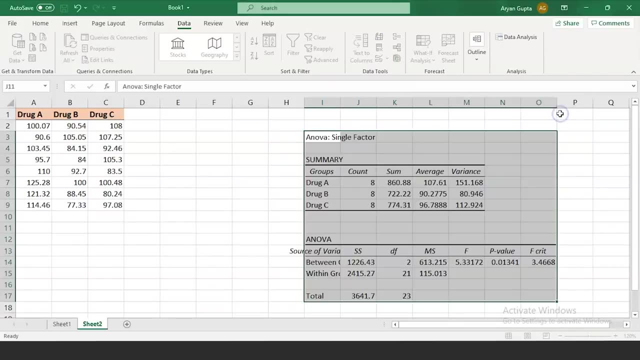 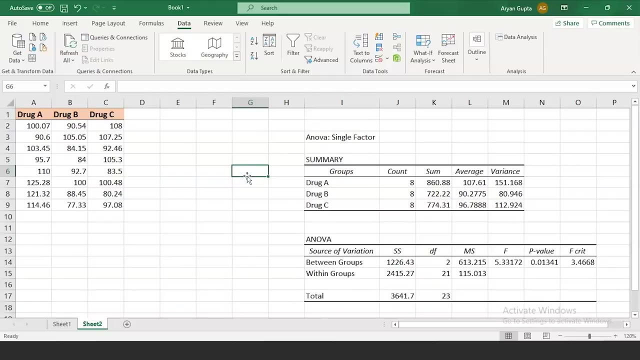 For the output range. We'll get the output here on the same page. So select some cell in the same page and we'll click OK, This is our output range. This is our group. So you can see. we have our analysis of variance table with the summary. 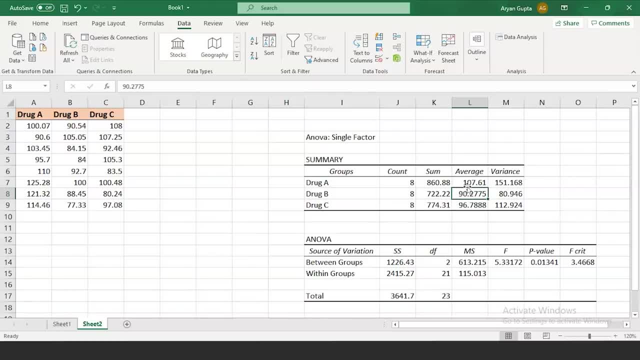 Let's understand each term one by one. The average time taken to cure the disease after consumption of 3 drugs are 107,, 90 and 96 hours approximately. The difference between the largest and the smallest mean is 17.47.. Here, one significant observation is that the F value is greater than F critical value.